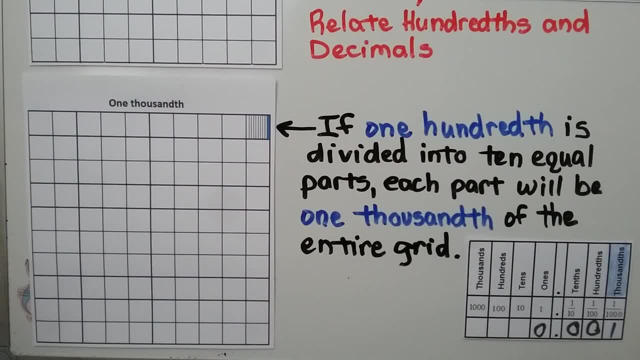 If one-hundredth is divided into 10 equal parts, each part will be one-thousandth of the entire grid. So here we split one of the hundredths into 10 equal parts. we have. the blue shaded area is one-thousandth. 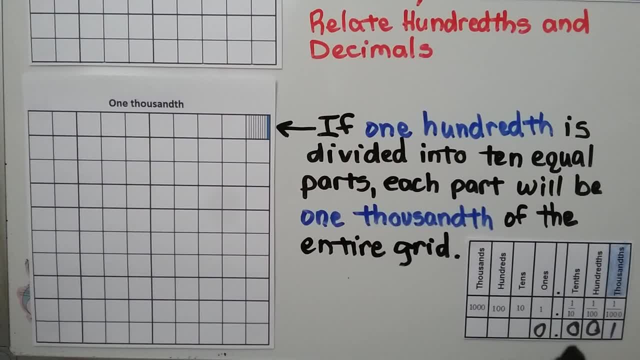 We would write it as a zero in the ones place, a decimal point, a zero in the tenths place, a zero in the hundredths place and a one in the thousandths place. There are ten times as many thousands as the hundredths. There are ten times as many thousands as the hundredths. 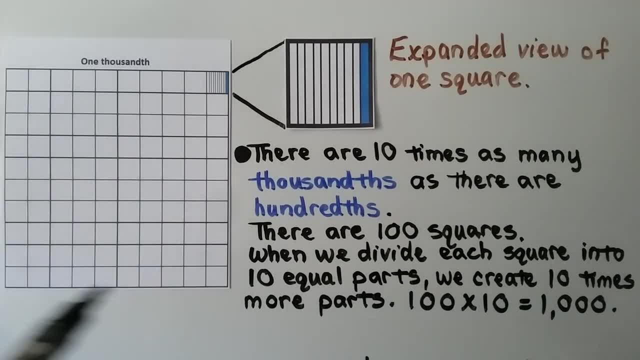 There are 100 squares here. When we divide each square into 10 equal parts, we create 10 times more parts. 100 times 10 is equal to 1,000.. If we split each of these squares into 10 equal parts like this, we would have 1,000 little parts. Each place value position is one-tenth. 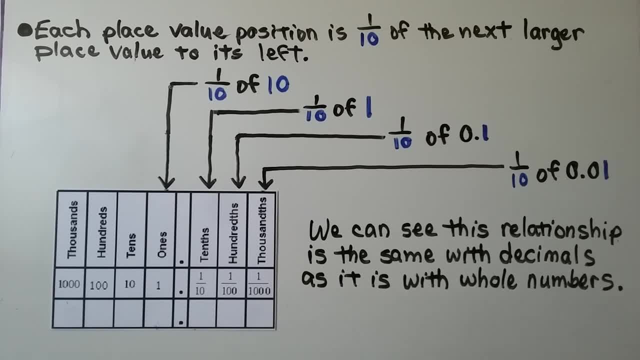 tenth of the next larger place value to its left. Here we have the ones: place One is one tenth of ten And for our tenths place one tenth is one tenth of one, One hundredth is one tenth of one tenth and one thousandth is one tenth of one hundredth, And we can see the relationship is. 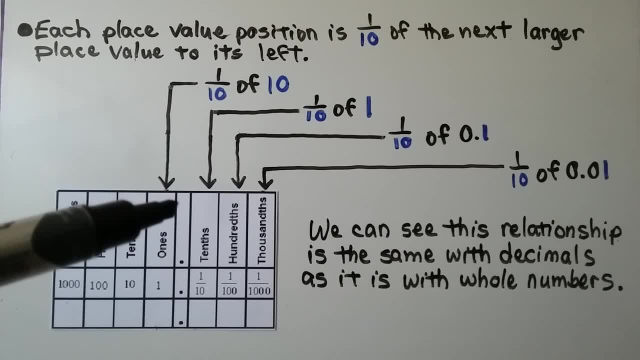 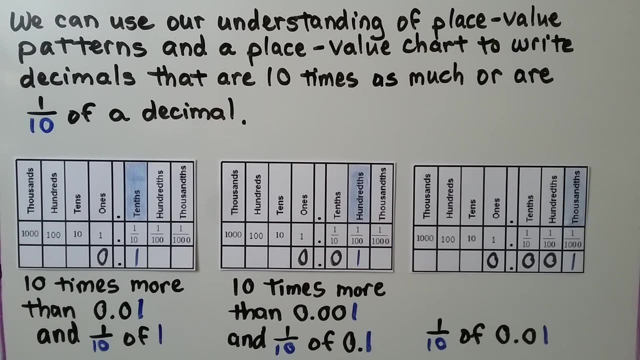 the same with decimals as it is with whole numbers. One is one tenth of ten. ten is one tenth of a hundred. one hundred is one tenth of a thousand. We can use our understanding of place value patterns and a place value chart to write decimals that are ten times as much or are one. 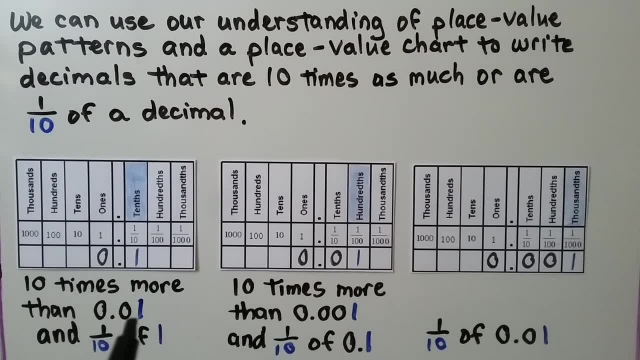 tenth of a decimal. Here we have one tenth. It's ten times more than one hundredth and it's one tenth of one. Here we have one hundredth. It's ten times more than one thousandth and it's one tenth of one. 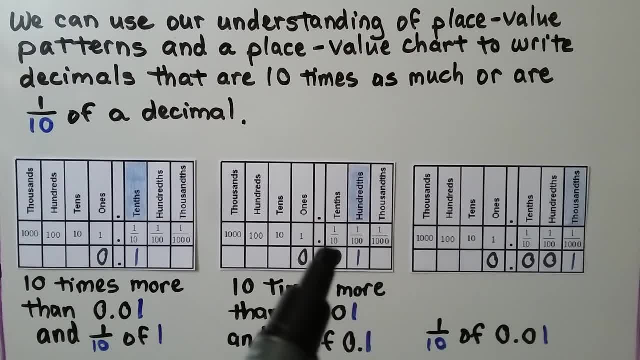 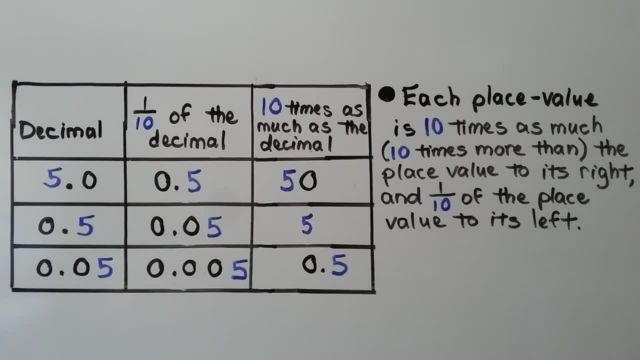 tenth And one thousandth is one tenth of one hundredth, So each place value is ten times as much. that means ten times more than the place value to its right and one tenth of the place value to its left. So if we look at the titles of our columns, we have decimal for the 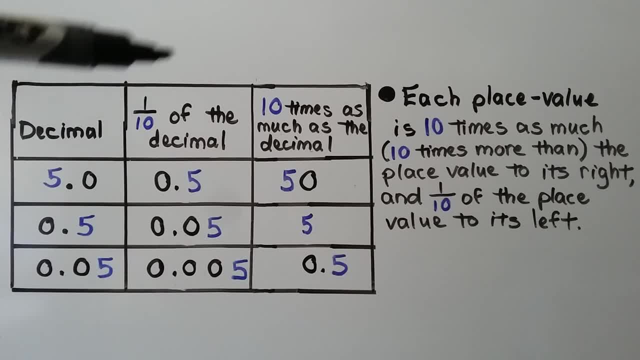 decimal number and one tenth of that decimal and ten times as much as that decimal. So our decimal is five and zero tenths, So it's just five whole. One tenth of this would be five tenths And ten times as much as five is fifty. Now we have five tenths for our decimal One. 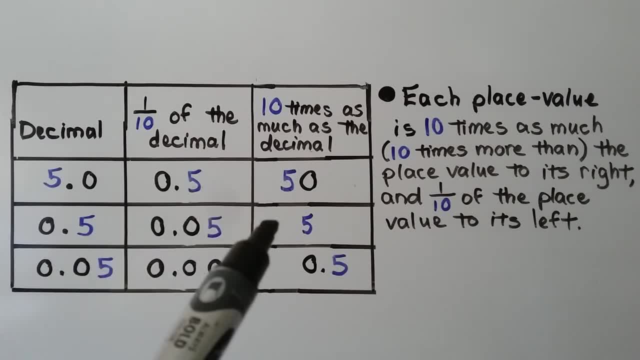 tenth of five tenths is five hundredths and ten times as much as five tenths would be five. Now we have 5 hundredths. 1 tenth of 5 hundredths would be 5 thousandths and 10 times as much would. 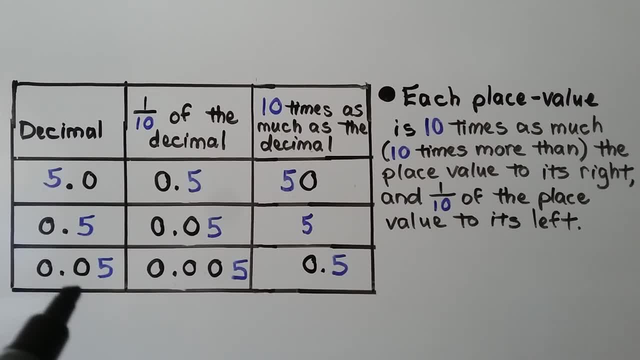 be 5 tenths And, if you notice, the decimal point is moving. Do you see how, for 5 tenths, 1 tenth of it, the decimal point moved to the other side of this 0? So now there's a 0 in. 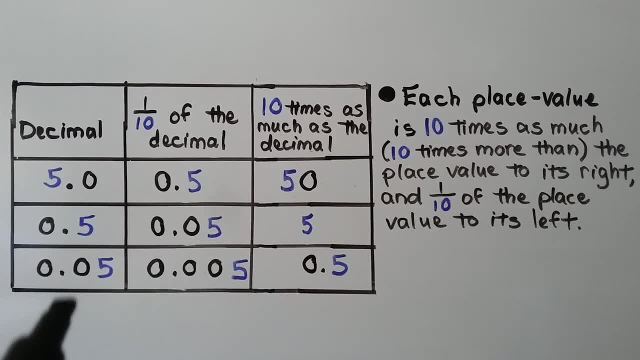 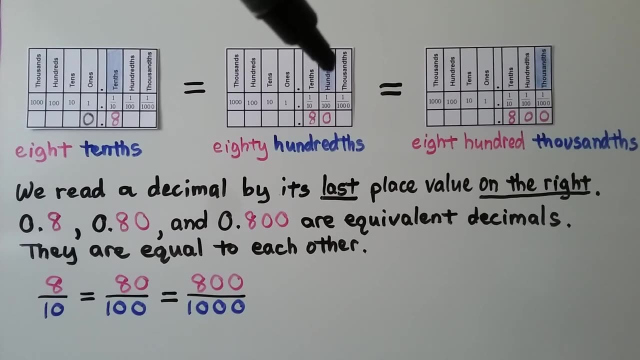 between the 5 and the decimal point, And here we had a 0 between the 5 and the decimal point, and now we have two 0s. See that Now we have none. Here we have 8 tenths, we have 80 hundredths. 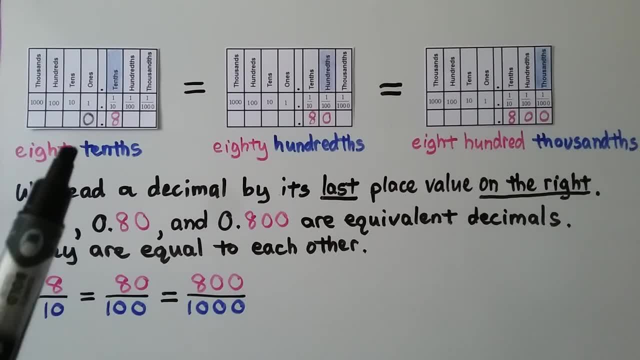 and we have 800 thousandths And they are all equal to each other. We read a decimal by its last place value on the right. So because the last place value on the right is in the tenths place, we read this as 8 tenths. If we put a 0 on the right side in the hundredths. 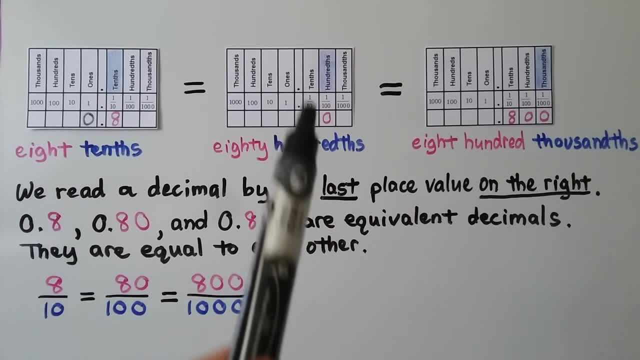 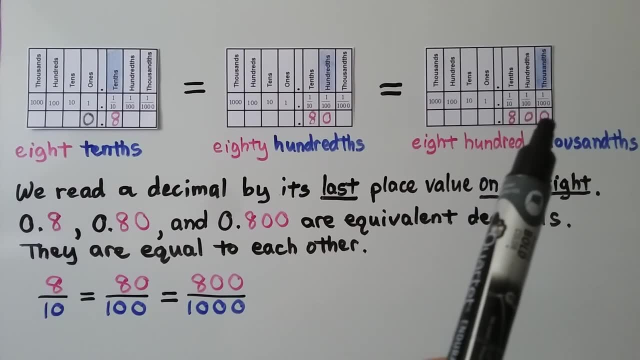 place, it's now 80 hundredths. But look, there's still an 8 in the tenths place. If we put two 0s on the right side now, its last digit is in the thousandths place, It's 800 thousandths. We still 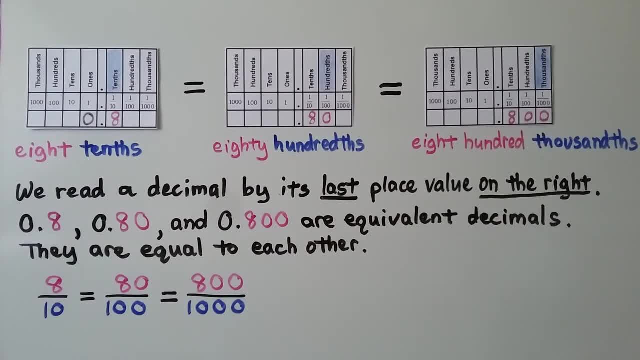 have an 8 in the tenths place, So 8 tenths, 80 hundredths and 800 thousandths are equivalent decimals. They are equal to each other. We can actually cover up the 0 in the numerator and the 0 in the denominator, or erase them and it. 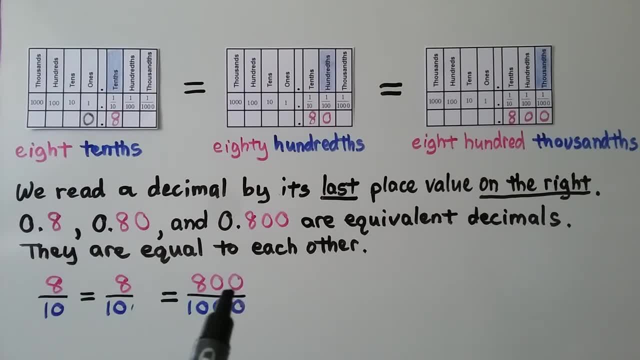 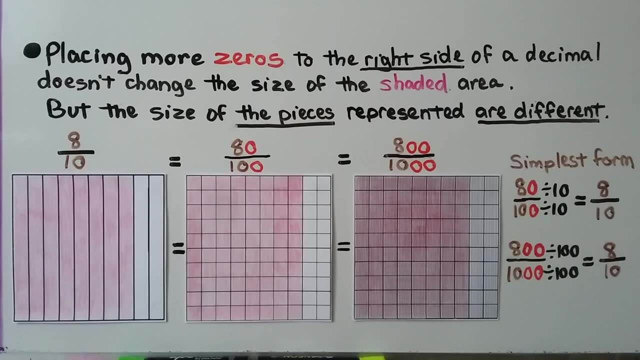 looks like 8 tenths, And if we erase the 2 zeroes in this numerator and the two zeros in this denominator, we have 8 tenths. That's actually what happens when we put them in simplest form, Placing more 0s to the. 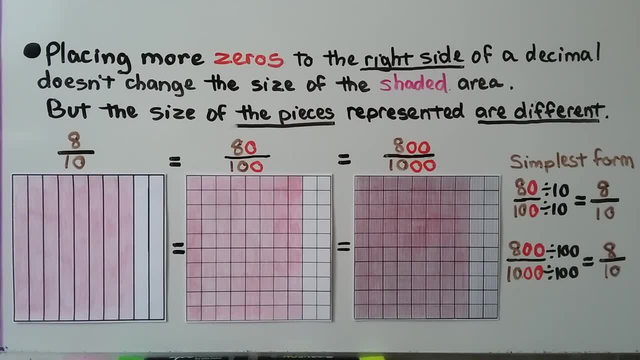 side of a decimal doesn't change the size of the shaded area. We have 8 tenths, so 8 out of 10 are shaded. Now we have it split into hundreds, so we have 80 out of 100 shaded. Now it's got very tiny. 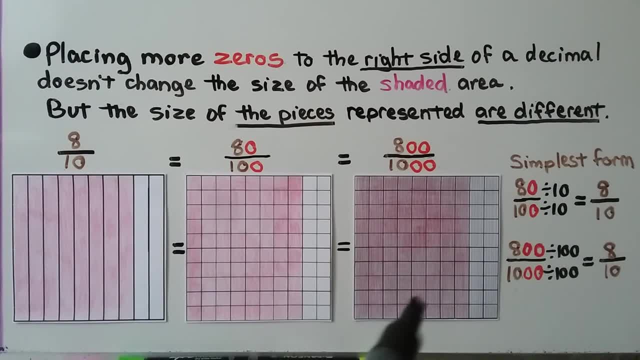 lines. We have 800 of a thousand shaded. We didn't change the size of the shaded area. It's the same amount that's shaded, but the size of the pieces represented are different. This is one big piece here, where it would be split into 10. here We have 10 big pieces split into 100 smaller pieces. 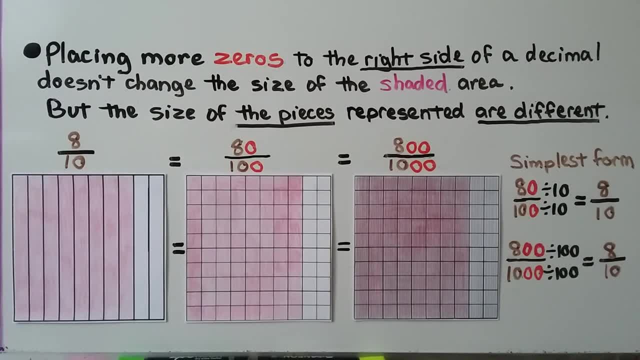 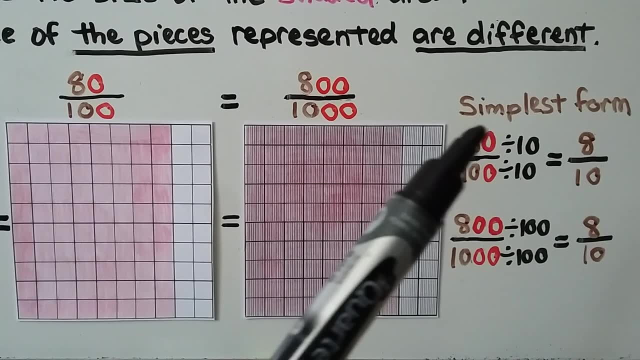 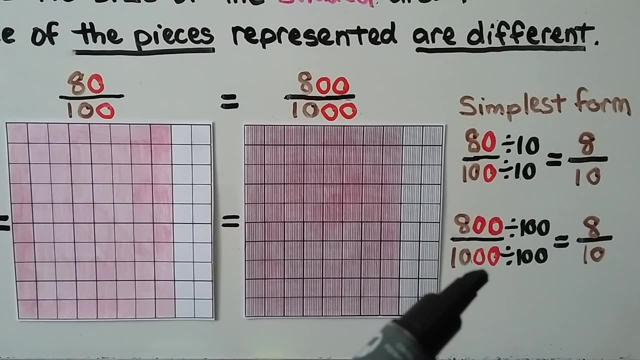 then they're split into a thousand, even smaller pieces. If we want to put 80 hundredths in simplest form, we divide the numerator and denominator by 10, and we get 8 tenths. And if we want to put 800 thousandths in simplest form, we can divide the numerator and denominator. 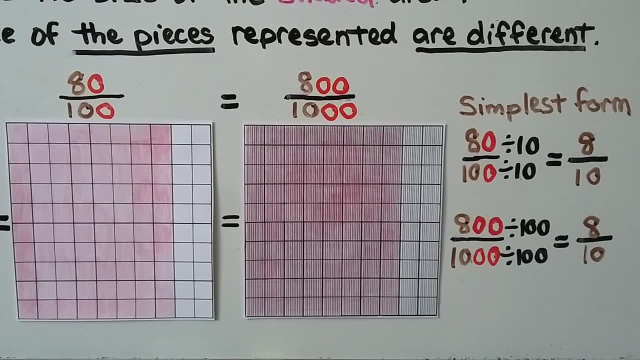 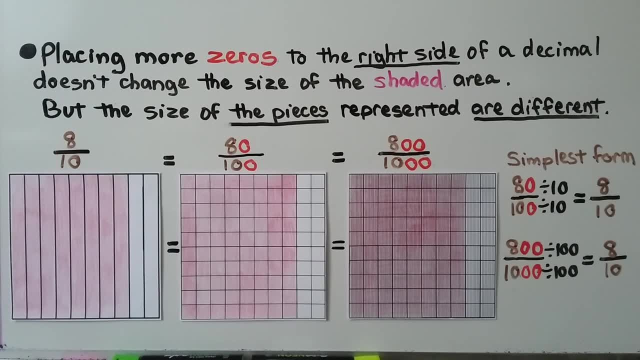 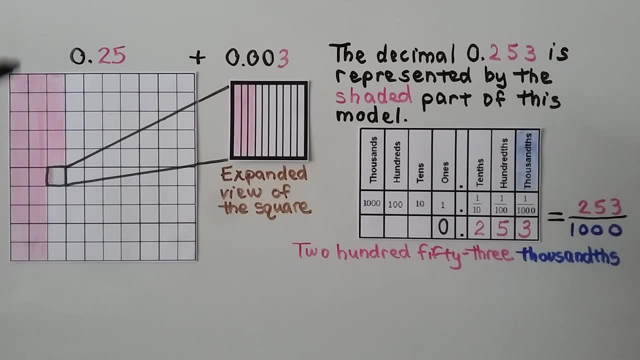 by 100, we get 8 tenths. We didn't change the size of the shaded area, but the size of the pieces that are represented are different. Here we have this grid and we have 10, 25 that are shaded in. Then we have this little piece. we have an expanded view of it. 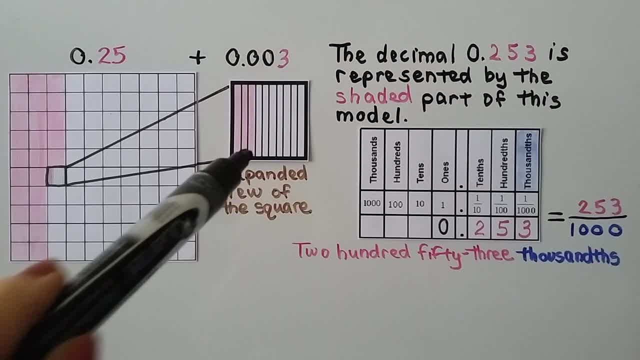 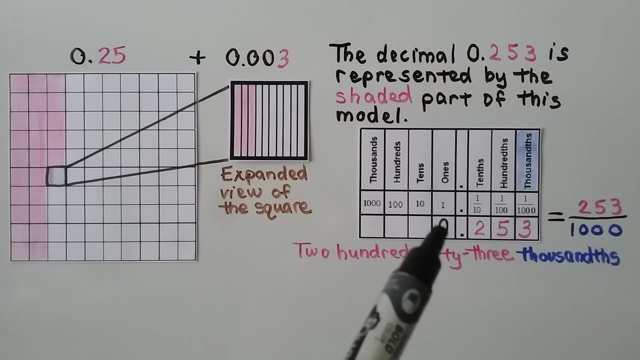 it has 3 shaded in here. These are hundredths, so these would be thousandths, And the decimal 253 thousandths is represented by the shaded part of this model. We have a 0 in the ones place, a decimal point, a 2 in the tenths place, a 5 in the hundredths place. 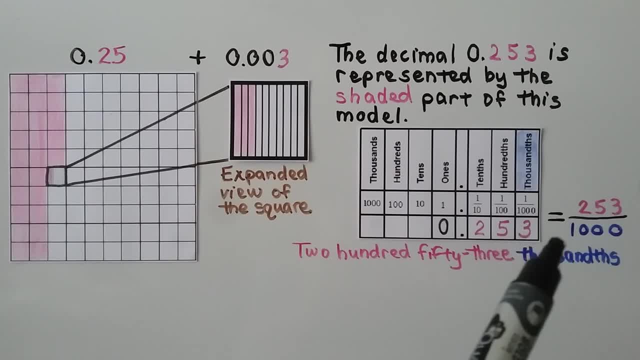 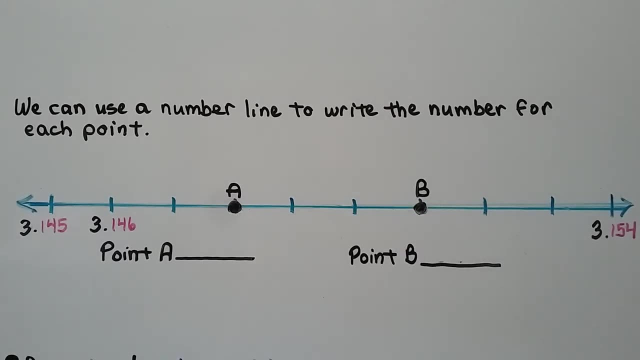 and a 3 in the thousandths place, It's equal to the fraction 253 thousandths. Here we have a number line with two points on it. We can use a number line to write the number for each point. We look on the left side and see it starts at 3 and 145 thousandths. 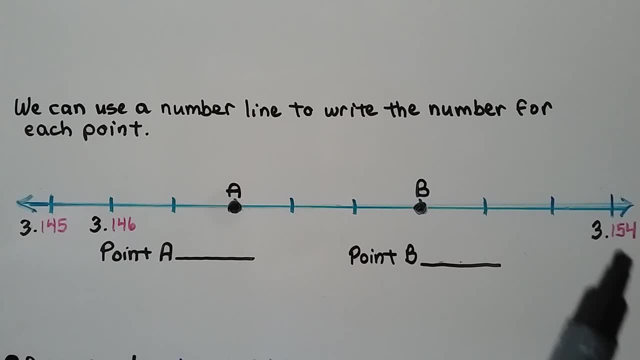 and over. here we have 3 and 154 thousandths. We can count or we could pencil in each increment to find where point A and point B are. Point B are on the number line. We have 3145 thousandths, 3 and 146 thousandths, so this would be 3 and 147 thousandths. 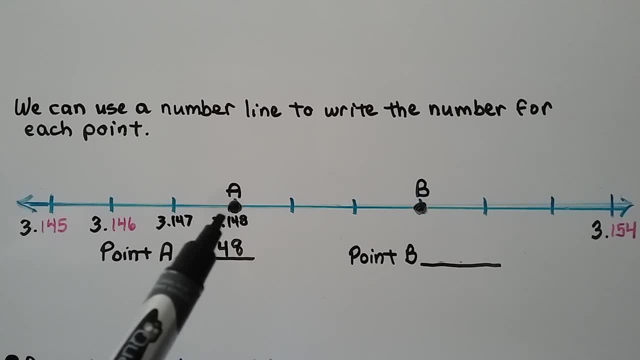 That means point A is at 3 and 148 thousandths. This would be 3 and 149 thousandths. We continue to count on by thousandths. We have 3 and 150 thousandths, 3 and 151 thousandths, and that is point B. 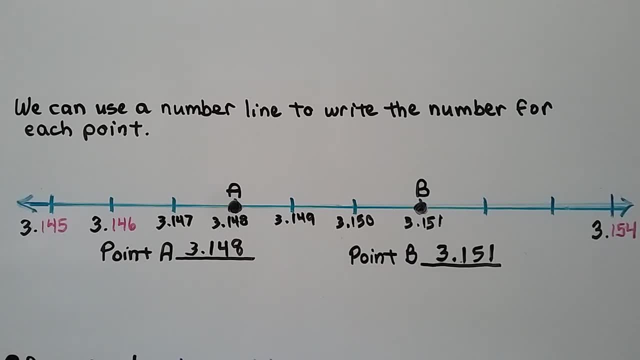 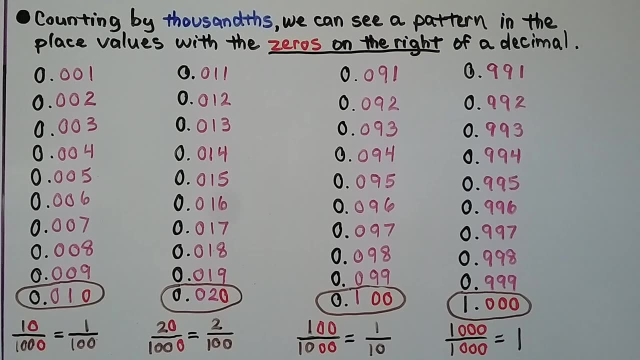 Point B is at 3 and 148 thousandths. This would be 3 and 149 thousandths. This would be 3 and 148 thousandths. Counting by thousandths, we can see a pattern in the place values with the zeros on the right of a decimal. 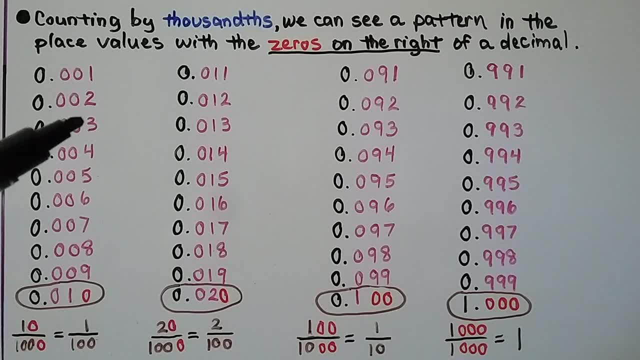 We start with one thousandth, two thousandths, three thousandths, four thousandths and we continue down to nine thousandths. Then we have ten thousandths. If we take this zero away from the right hand side, we see it's one hundredth. 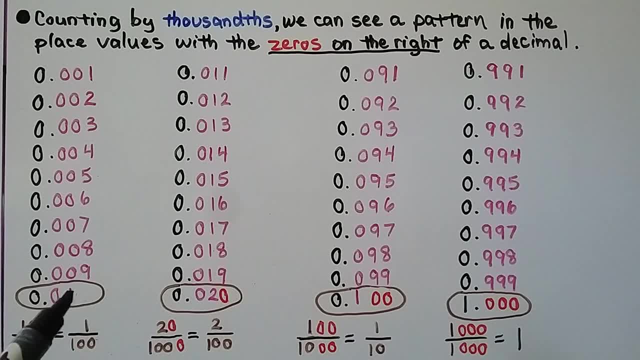 If we take this zero away from the right hand side, we see it's one hundredth. Then thousandths is equal to one hundredth. We just put a zero there. Here we have eleven thousandths, twelve thousandths, thirteen thousandths, fourteen thousandths. 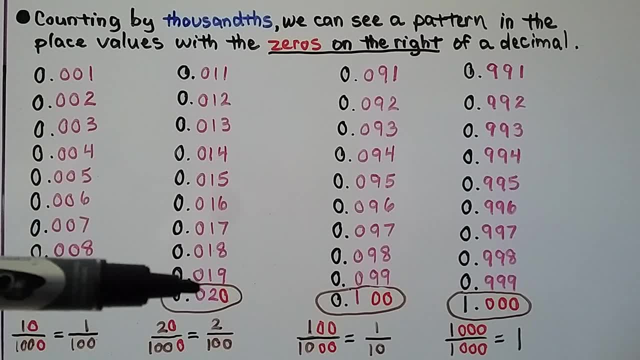 We go all the way down to nineteen thousandths, and the next one would be twenty thousandths. We can take away this zero on the right hand side and it's two hundredths. Twenty thousandths is equal to two hundredths. Now let's skip up to ninety-one thousandths, ninety-two thousandths, ninety-three thousandths, and we go all the way down to ninety-nine thousandths. 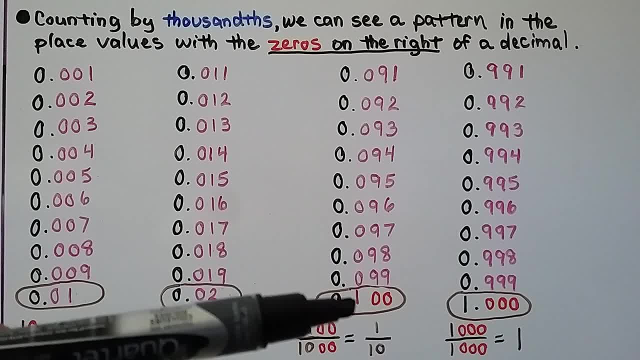 The very next number would be 100 thousandths, We would have one hundred thousandths And if we took the two zeros away on the right hand side, we have one tenth. If we jump to 90 and 149, we get nine thousandths. 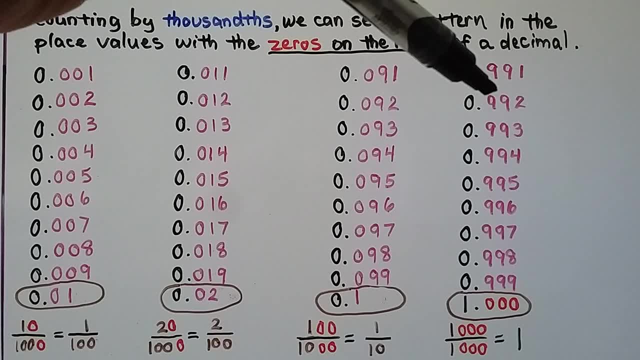 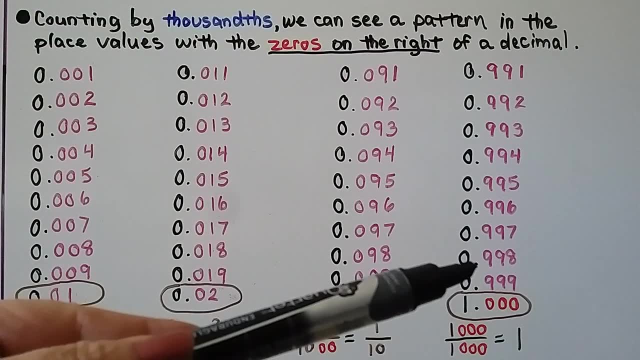 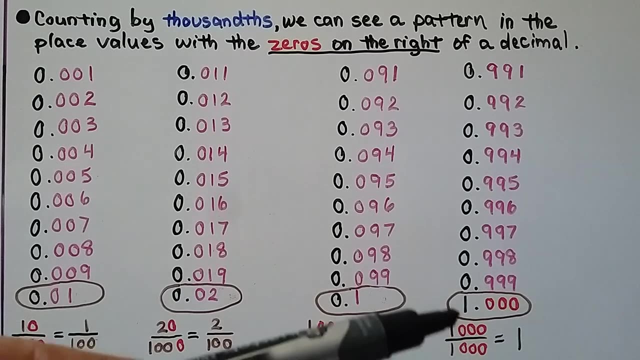 991 thousands, 992 thousands, 993 thousands and we go to 999 thousands. the very next number would be 1000 thousands. we have the same numerator and denominator. if we had something split into a thousand pieces and we had all 1,000 of them, we would have the whole thing. it would be one whole and we can. 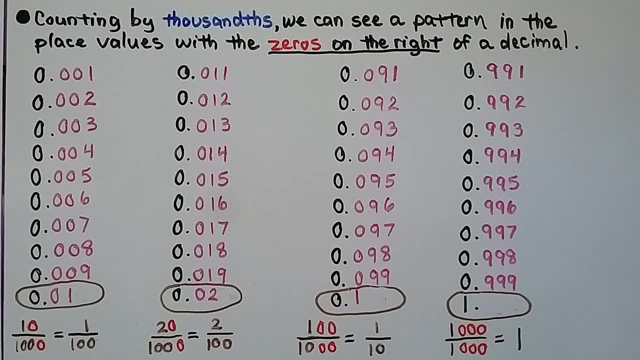 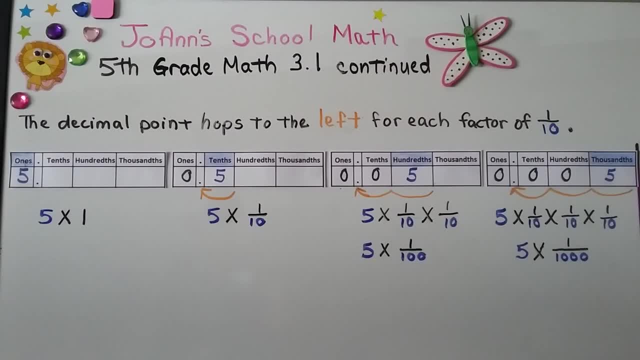 take away the zeros on the right hand side and see it is one one whole. the decimal point hops to the left for each factor of 1 10th. here we have 5 whole, that's 5 ones. now we have 5 tenths and the decimal point went from this side on. 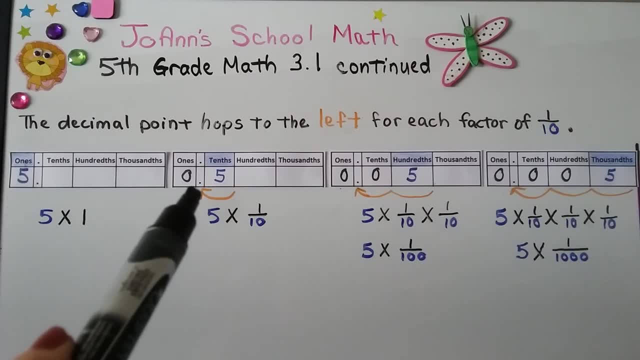 the right side of the 5 whole ones to now it's on the left side, so it made one hop to the left. and now it's on the right side, so it made one hop to the left. when we multiply the 5 whole times 1. 10th, when we multiply the 5 times 1: 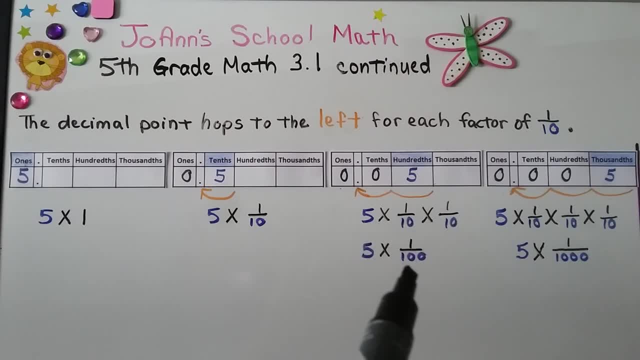 10th times 1 10th. 1, 10 times 1: 10th is 1 hundredth, isn't it? for each factor of 1, 10th, the decimal point is going to hop to the left, so it's going to hop once. 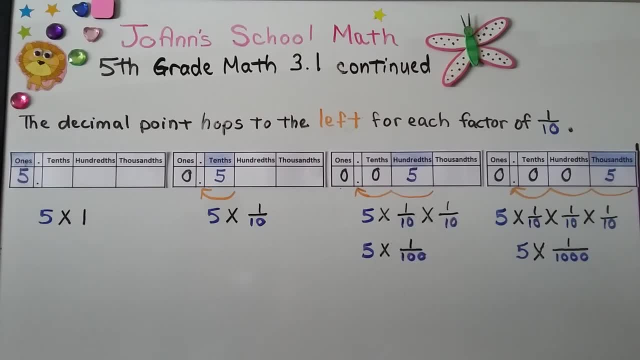 twice for each factor of 1- 10th. now we have five hundredths. that's five times 1, 10th times 1, 10th times 1- 10th. that means that decimal point is going to hop three times. it's going to hop 1, 2, 3 times and 1- 10th times 1, 10th times 1. 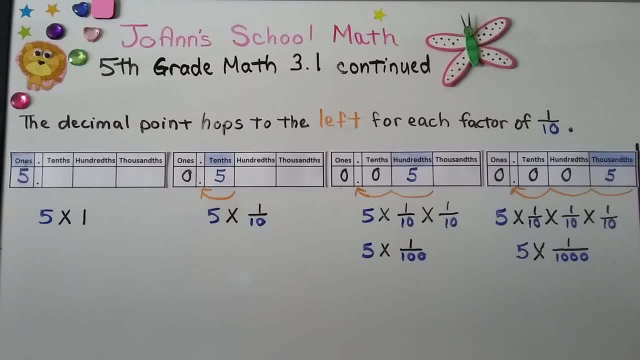 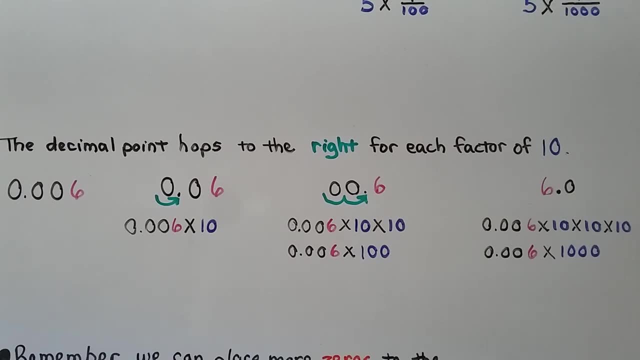 10th is 1 thousandth, so that would be the same as 5 times 1 thousandth. the decimal point hops to the right for each factor of 10 whole. here we have 6 thousandths. if we multiply 6 thousandths times 10 whole, we move the decimal point from. 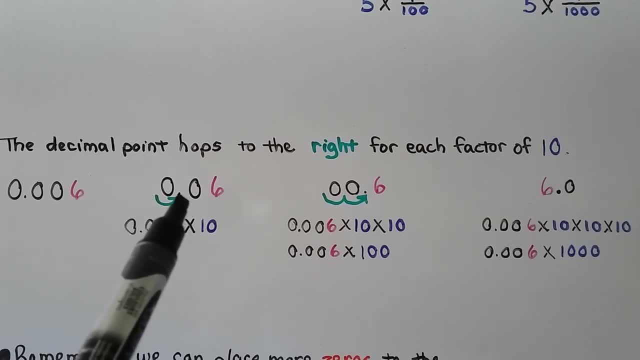 this side of this 0 to here, now we have 6 hundredths. and if we multiply 6 thousandths times 10 whole times 10 whole, we're going to move the decimal point to here: 6 thousandths times 100. and if we multiply 6 thousandths times 10, 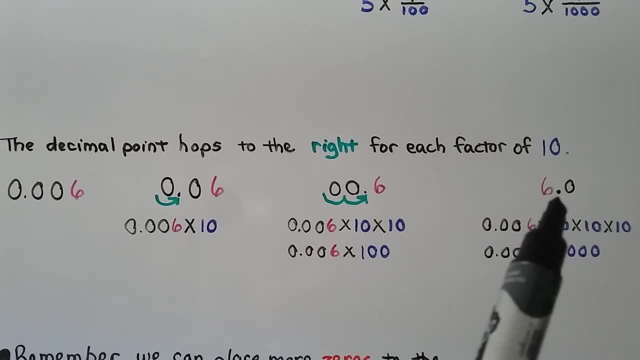 times 10. times 10, we move the decimal point to here. The decimal point moved to the right one hop for each factor of 10.. By multiplying 6 thousandths times 1000, we have 6 whole. So remember we can place more zeros to the right side of a. 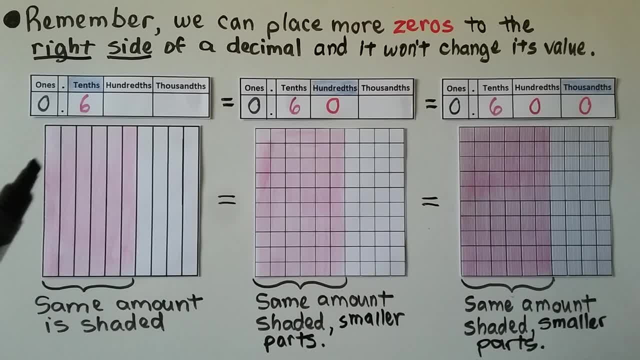 decimal and it won't change its value. 6 tenths is equal to 60 hundredths, which is equal to 6 hundred thousandths. The same amount of area is shaded. they just have smaller parts. These are smaller parts than tenths and these are smaller. 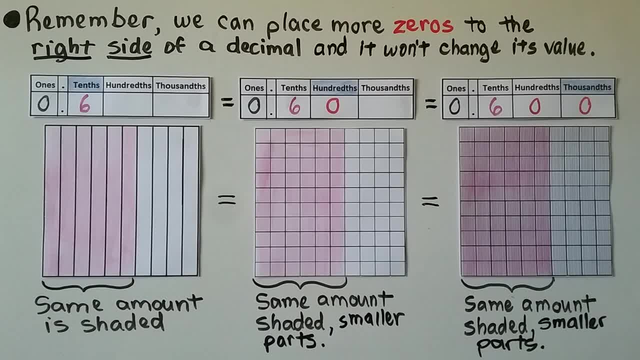 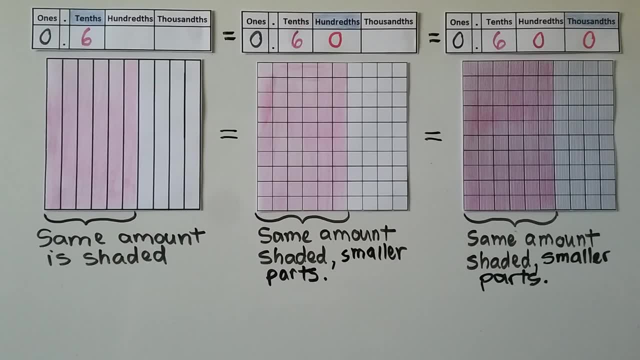 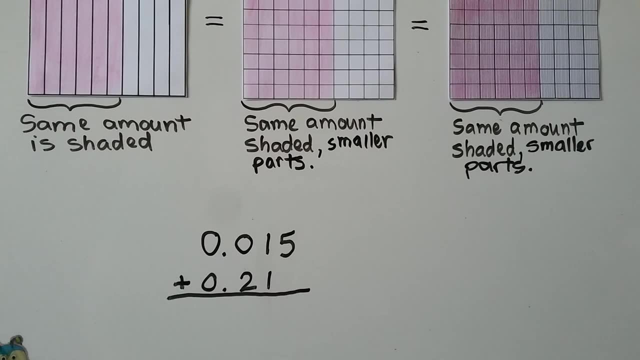 parts than hundredths. Adding zeros to the right side of a decimal is very useful when we're adding a question. Sometimes when we add decimals, there'll be an empty space here and we could put a zero there as a placeholder. It doesn't change the value, but it helps us to add. 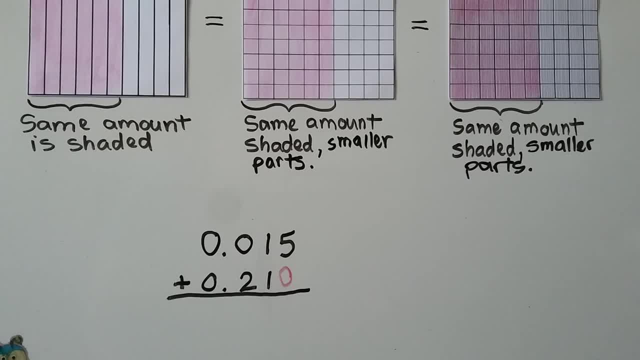 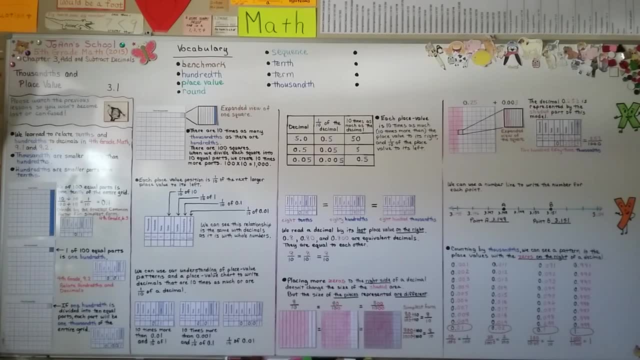 our columns. We'll talk about that more in a few lessons. In our next lesson 3.2, we're going to talk about place value for decimals, for tenths, hundredths, thousandths, and how to read and write them in standard form, word form and expanded form. I hope I'll see you there and I